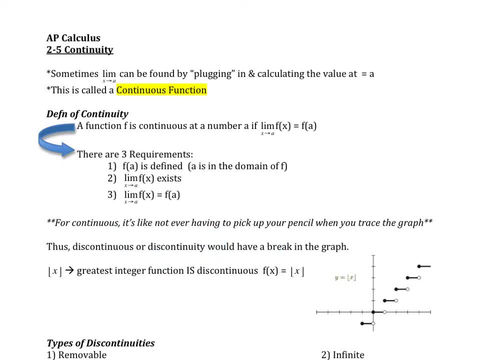 So that's how you can do it graphically, As long as you can trace the whole function. so suppose I had something that looked like this And I had some function that came up, came down, came back up, whatever, I can take my pencil- or my lightsaber in this case- and trace the whole thing without ever having to pick it up. 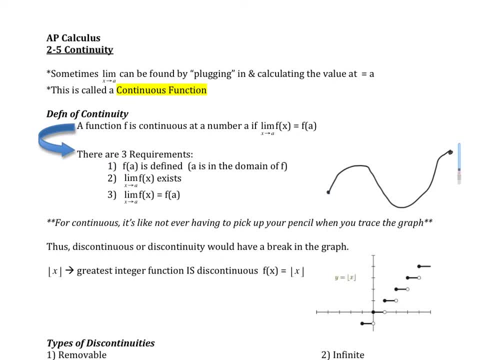 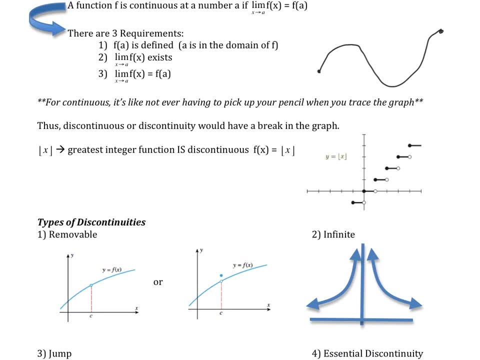 Then that means it's continuous. Now you can have continuity on an interval or you can have continuity for the whole graph itself. So let's take a look here: If we have this absolute value function- I'm sorry, this greatest integer function, 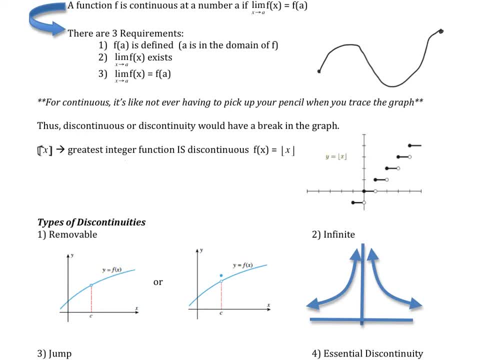 and this obviously my software doesn't do it right, so it should look like this: okay, And I graph this greatest integer function. I will get this step function. Notice how this step function is not continuous, because to go from here I have to pick up my lightsaber and then go here. 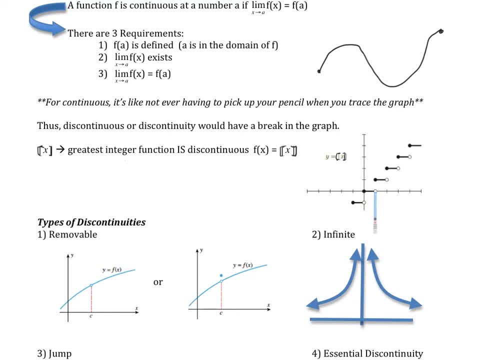 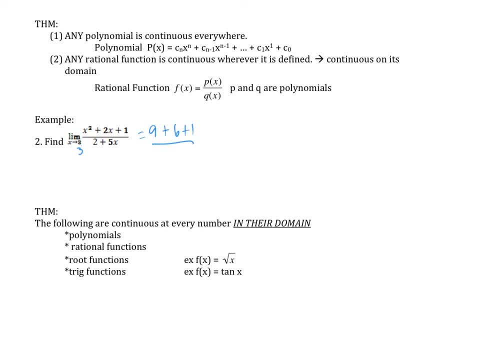 So as long as you can trace the whole thing without ever having to pick it up, you're good to go Over here. the following are continuous at everywhere in their domain. We said polynomials, We said rational functions, We saidnent and root functions are also continuous everywhere in their domain. 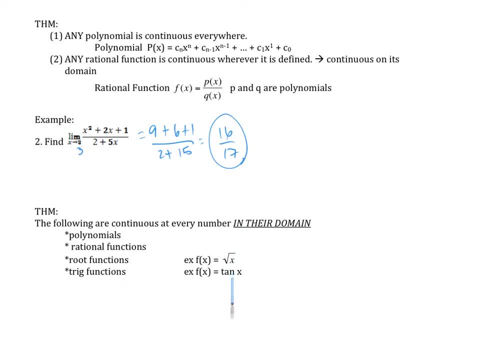 And trig functions will be continuous everywhere in their domain. Root function and example would be the square root of x and a trig function and example would be tangent of x, continuous in their domain. be careful, I'm just saying in that domain. Alright, let's move on. 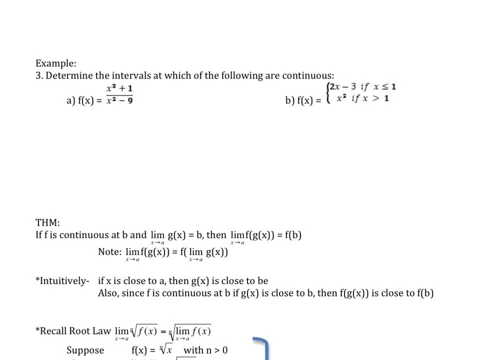 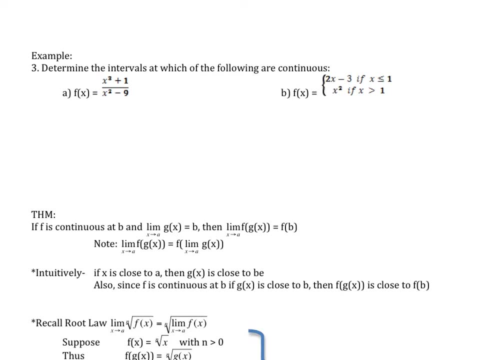 So now we have over here our third example: determine the intervals of which of the following are continuous. So this first one is a rational function. so I need to determine what the domain is and it's continuous in that domain. So if I take a look at this graph, we'll do it graphically on this one. 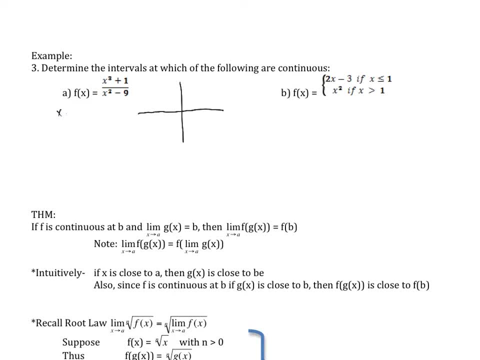 You can have also done it by hand, and just note that you have asymptotes at x equals plus or minus 3, right? And so we are going to have these asymptotes, and if you graph it with a calculator, that's good as well. 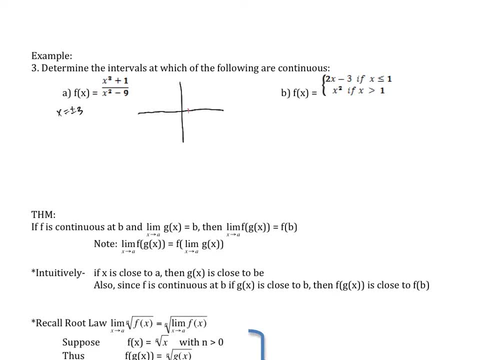 But anyway, you will have asymptotes at x equals plus or minus 3, right There and right there, And this graph will look like this: in between those, This is one of those that does this funky thing like this, and then, on this side, you'll. 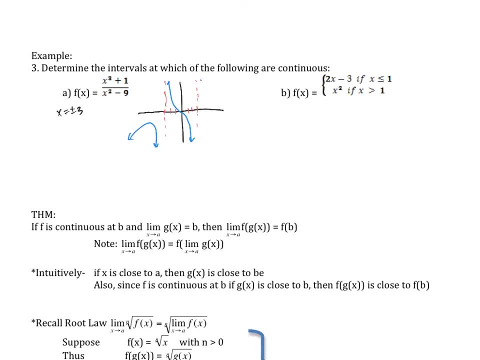 have something that looks like this, and on this side it will follow the asymptote up and then go like that: Alright, so we need to determine where it's continuous Over here. well, we cannot use. we could say: the domain is all reals except x equals plus. 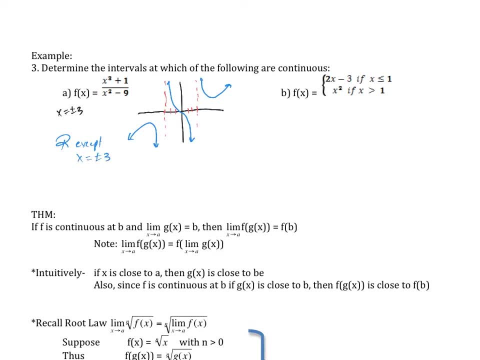 or minus 3, right, Because we have asymptotes there, So it's continuous from negative infinity to negative 3, and so we're going to do the union symbol negative 3 to 3 and from 3 to infinity. And notice, I did not include these because those are asymptotes. 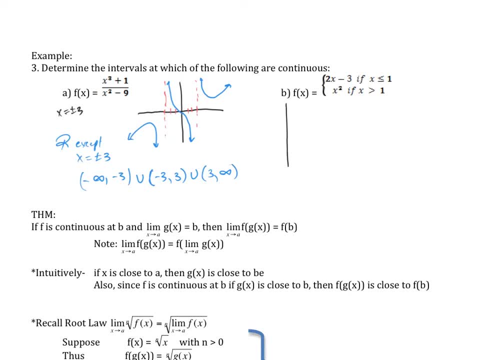 So now let's take a look at this next one. Let's sketch a graph of this real quick so we know what we're looking at, And over here I have this equation: when x is less than or equal to 1, and I have x squared when x is. 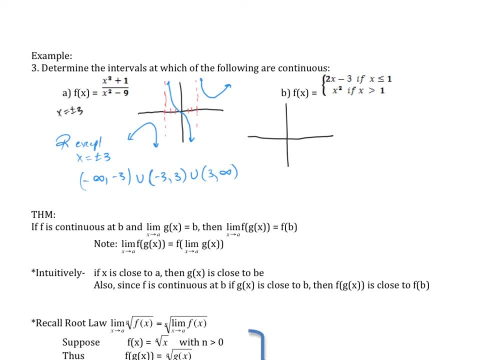 greater than 1.. So something happens at 1.. That is my border, so to speak, And over here it's x squared, so it'll be from right here and this will go up, And on the other one it's 2x minus 3.. 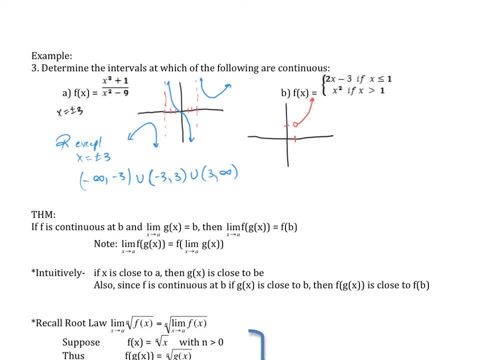 So when you put in 1, you're going to get negative 1.. So it's right here and that's an equal to it. When you put in 0, you'll get negative 3.. So this one looks like this and it's linear. 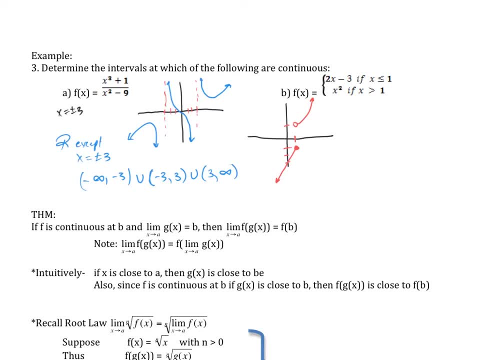 Alright, so now we know what we're looking at. So right here, even though we have two polynomials, our point in question is this: At x equals 1.. First of all, let's look at the three parts of continuity. First of all, does f of x- in this case it'll be f of 1, f of a. 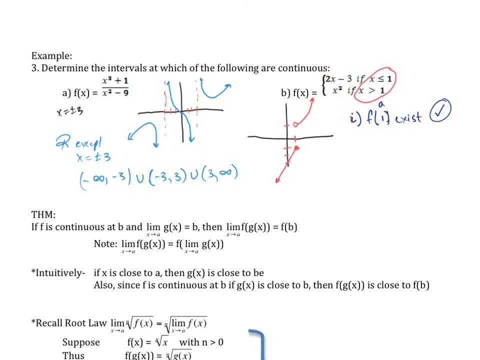 Exist? Yes, it does exist. F of 1 will be this value right here at negative 1.. Does the limit as x approach 1 exist? So when I come in from the left- that's this one- I get negative 1.. 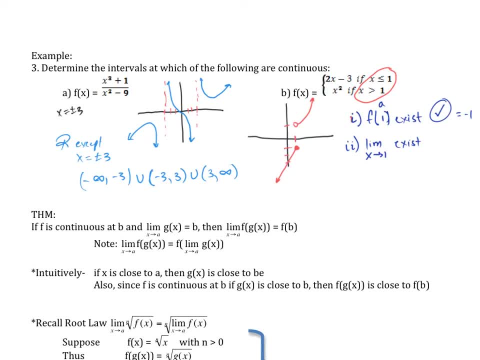 When I come in from the right, I get positive 1.. So this is no, it does not. So that means I don't even have to. I don't even get to step 3.. And we even know by just looking at the graph: there's a discontinuity at 1.. 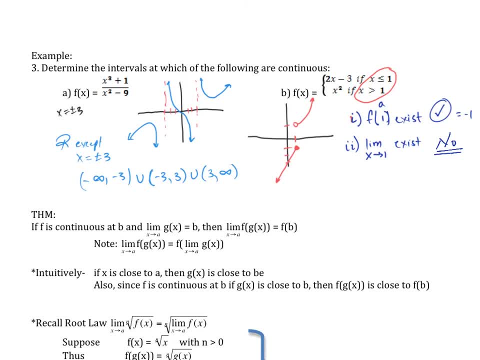 So the only spots that this is continuous that I can say is from negative infinity to 1, like this: That's this part of the graph- And from 1 to infinity. So I cannot take that discontinuity Into play. So that's how I have to write this. 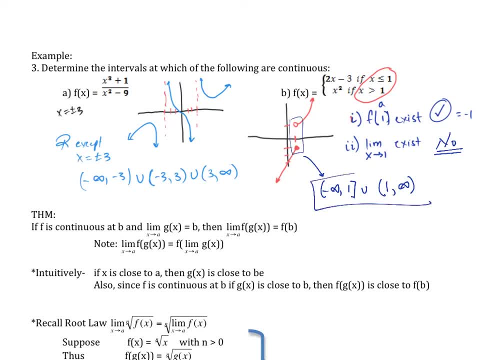 Because there is a discontinuity that occurs right there. Alright, So now we have this other theorem: If f is continuous at b and the limit as x approaches a of g of x equals b, then the limit as x approaches a of f of g of x equals f of b. 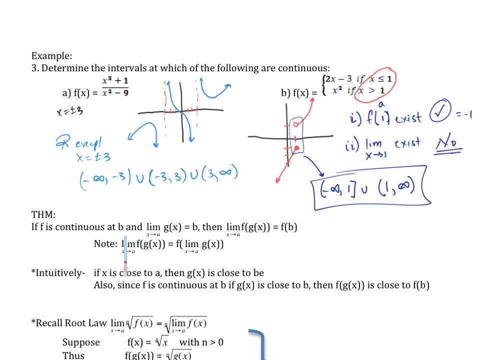 So this is the compositions, So I can actually take the f composition out and do this So intuitively: as x gets, as x is close to a, Then g of x is going to be close to b, not b, e, b. 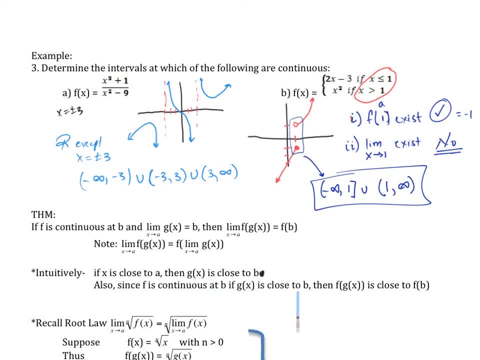 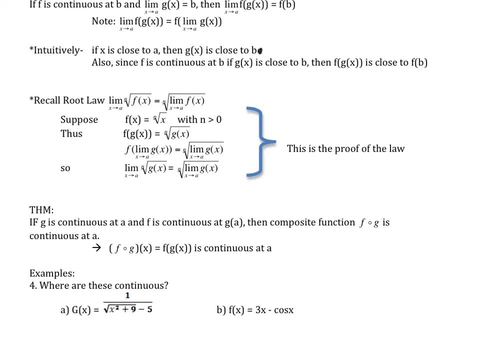 Also, since f is continuous at b, If g of x is close to b, Then f of g of x is also is close to f of b. Then we have this: that develops the root law, And the proof of this law is in your book. 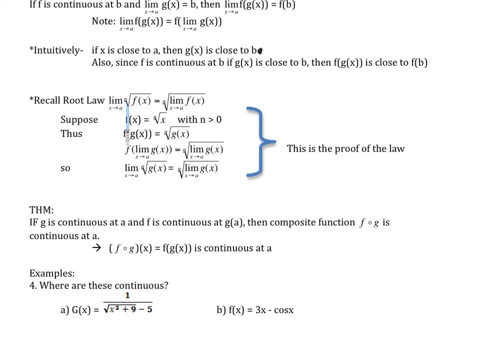 I'm not going to go through it, But just know that the limit as x approaches a of the nth root of some function. You can take that outside. Take the limit of the function, Then take the nth root of it. So that's what this one tells you. 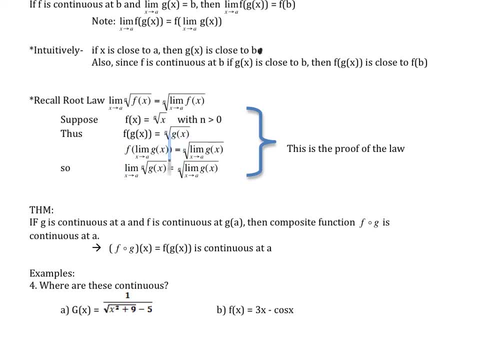 And it's here is the proof of it, But I'm not going to go over that And you don't really need to know it in detail. So if g is continuous at a And f is continuous at g of a, Then the composition f of g is continuous at a. 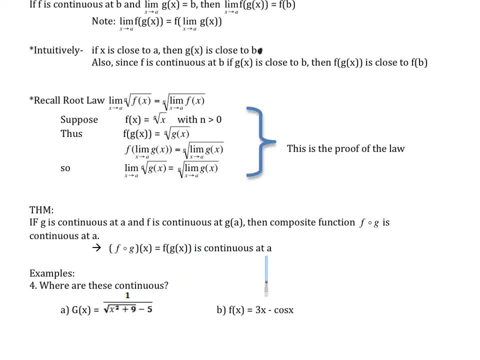 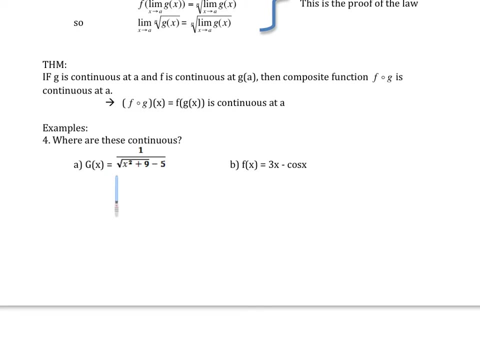 So f of g of x, f of g of x will be continuous at a. So what this is saying is compositions, as long as this is continuous, will be continuous as well. I'm going to save these two examples for class. Your author likes these a lot. 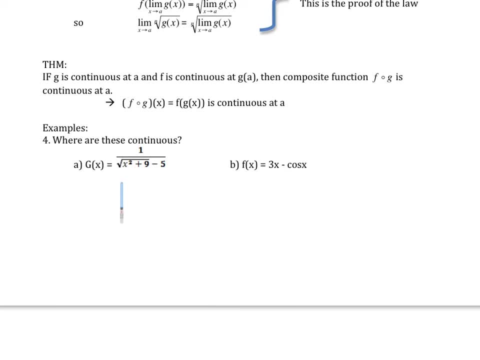 And basically all you're trying to do on these is do compositions to show that, well, this is continuous, So the other thing has to be continuous And same with over here. But I'm going to do these in class. In fact, I'll just do this one right now, since it's a little bit easier for you guys. 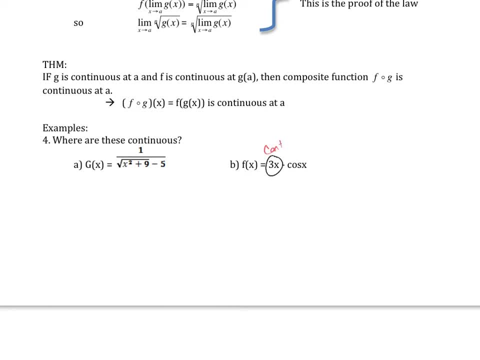 This is continuous. Let's do it like this: Right, That's a polynomial, This is a trig function. This is continuous. So if I have continuous minus continuous, one of the laws told me that it will be continuous, So it'll be continuous on all real values, because this is continuous on all real values. 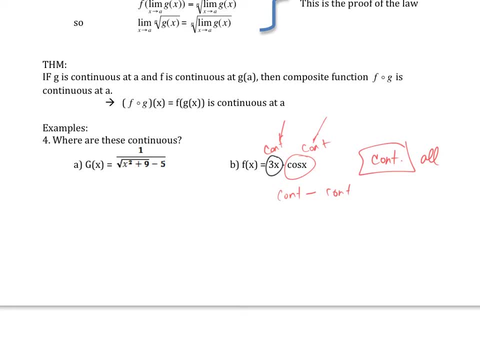 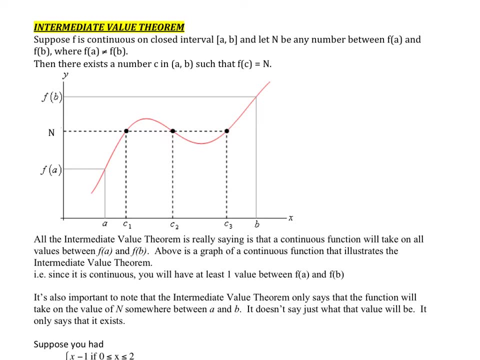 And that's continuous on all real values as well. All right, Let's move on. Take a look at the next thing, which is IVT. At this point in the lesson, I would recommend that you pause, go, take a break, just hang. 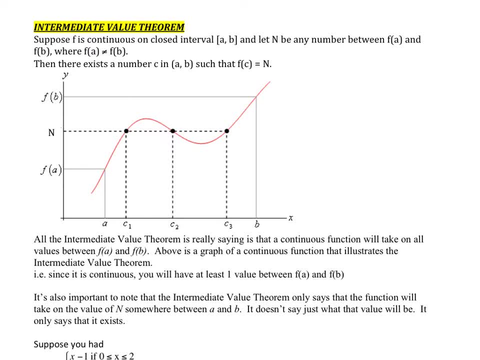 out a little bit Because catch your wind, Because this is another biggie, So I need your full attention for this one. All right, So the intermediate value theorem, commonly abbreviated as IVT- super important- Typically does show up on an AP test. 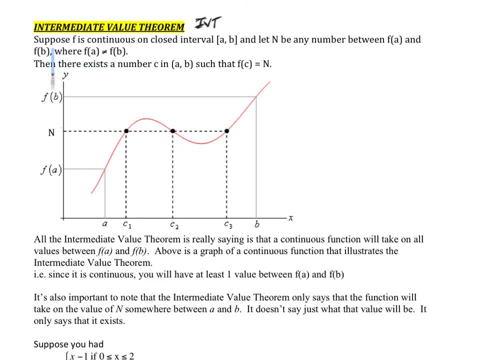 And let's just read what the definition is. first, And I'll explain all this to you: Suppose f is continuous on a closed interval a to b. So it's a closed interval from a to b And let n be any number between f of a. 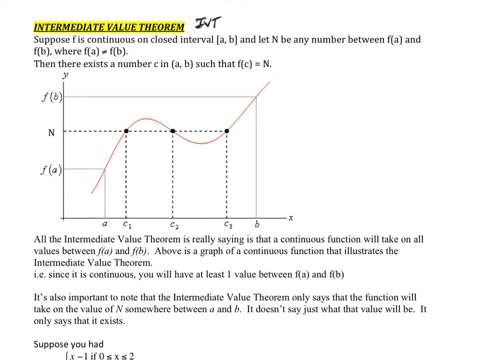 And f of b, where f of a doesn't equal f of b. So we have the sum number on a closed interval, a corresponding to f of a And b and f of b that correspond. Then there exists a number c in a- b, such that f of c equals n. 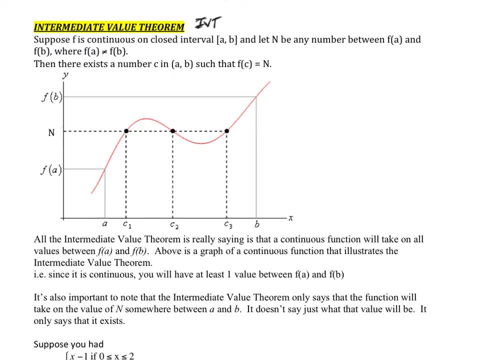 All right. So the intermediate value theorem is really saying that a continuous function, no matter how you draw this, will take on all the values between f of a And f of b. So if it's continuous, there's going to be values all in between here. 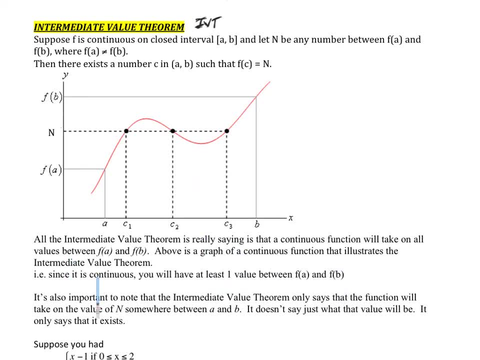 So this graph shown illustrates the IVT. Since it is continuous, you will have one value between f of a and f of b. So here's a, Here's what IVT says, Think intermediate. Here's a, There's b. 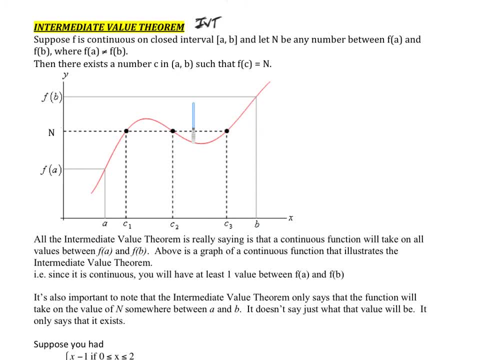 If you have something in between, so this would be f of a, This would be f of b And f of a, And you put something in between a and b. well then this has to be between this n value, has to be between f of a and f of b. 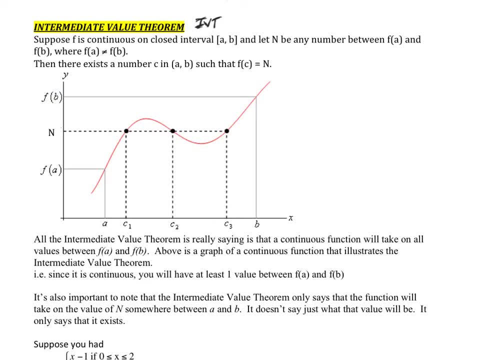 It's pretty like logical thinking. Now here's another example I can give you. Suppose this is your house right here And here's school And here's your friend's house. If you're going from your house To your friend's house, 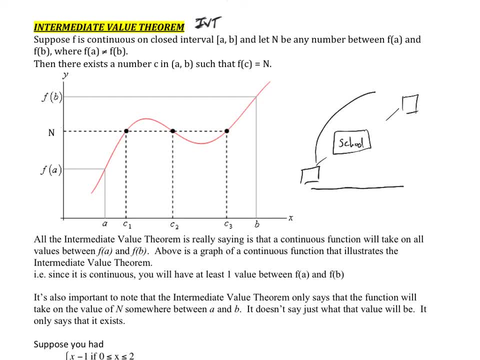 No matter how you go, You can go up and around. You can go this way and around You can go this way. then up, You're going to cross the line where school is. Now I know some of you are saying, well, I'm going to go all the way around the world. 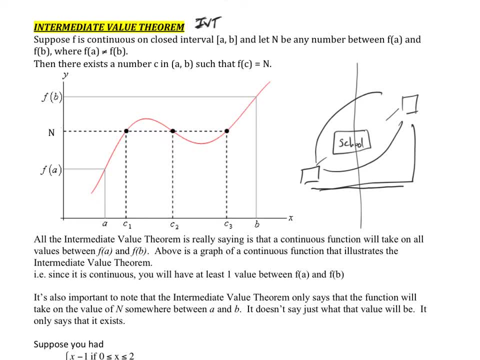 Okay, you go ahead and do that, But to demonstrate IVT, To get from point a to point b, From your house to your friend's house, You're going to have to cross this line where school is at. And you're going to have to cross this line where school is at. 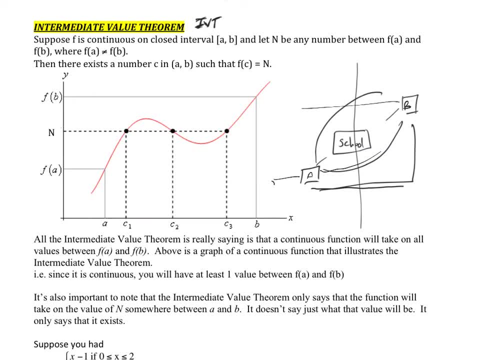 And once you do that, That means you'll have some value f of a here, Some value f of a- b there. Once you cross that line, You will have some value here that we will call n On the y axis. Now it's important to note that the intermediate value theorem 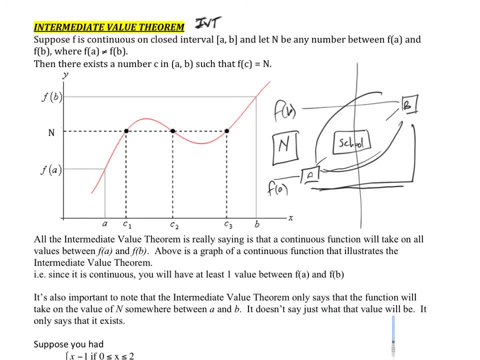 It only says the function will take on some n somewhere. It doesn't say what the n will be. It only says that it has to exist. But remember what the conditions are. The conditions are: it has to be on the closed interval And it has to be continuous. 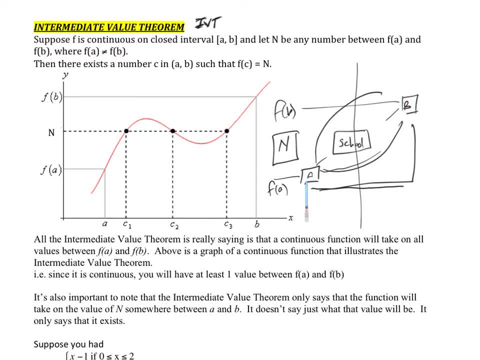 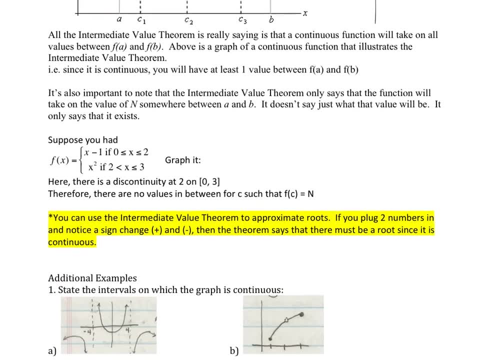 So it has to be continuous from here to here. You can't just jump around, Then you'd have a discontinuity. IVT obviously wouldn't work, And so let's look at this example for that, And again, they will present these in various ways. 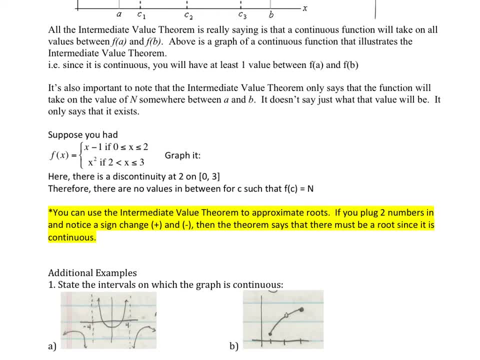 And we'll show you the ways And I'll show you all the different ways that they would present them on the AP test. But let's look at this one right now. Right here it says graph this: Okay, So suppose we had this situation. 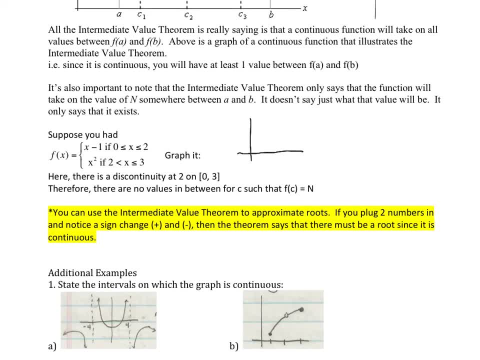 I'm going to go ahead and graph it for you right there. And from 0 to 2 you have this equation for: and it's x minus 1.. So when I put in 0. I will get negative 1.. And let's graph that. 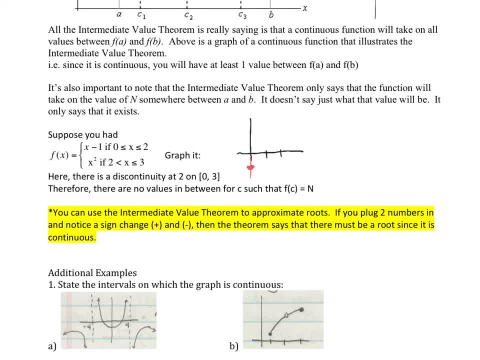 So that's down here at negative 1.. And then when I put in 1, I obviously get 0. Okay, And at 2 I'll get a value of 1. And this is equal to it here and here. So these will be closed and it looks like this: 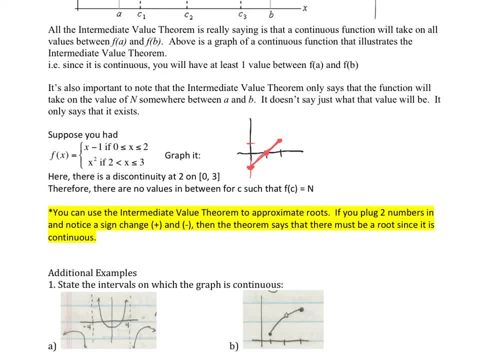 Now the next part of the graph is x squared Whenever x is between 2 and 3.. So here's 2, 3. And this is x squared. So when I put in 3, I come all the way up here to 9.. 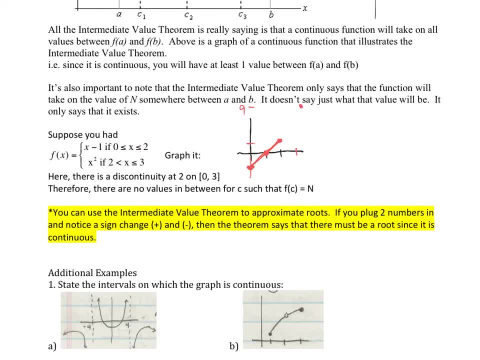 We'll just kind of exaggerate that, because it's not perfect right there. And when I put in 2. I'm going to get a value of 4.. Okay, And I'll 1,, 2,, 3,, 4, and this is a break in the graph because it's not a perfect graph. 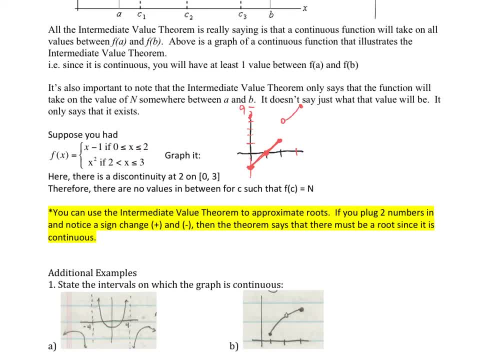 here. I didn't have enough room to draw it, So that's an open circle and it looks parabolic in nature like that. All right, So does IVT work here? No, There's a discontinuity. I can't follow from here to there without when I get here, I got to jump up. 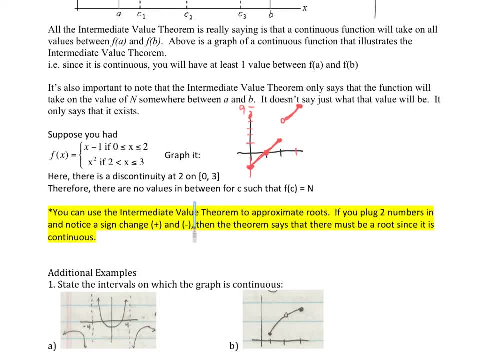 There's a jump discontinuity there, So IVT wouldn't hold. So therefore there is no values in between for c, such that f of c equals n. Here's how we used to use intermediate value theorem a long time ago. Your calculator is doing a little different now. 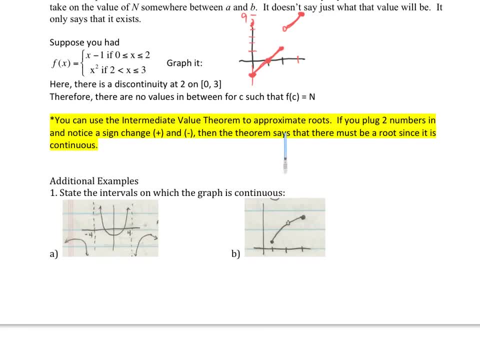 But IVT. you can use IVT to approximate roots. If you plug two numbers in and notice a sign change between positive and negative, then the theorem says that there must be a root as long as it's continuous. So wait, Let's see what that means again. 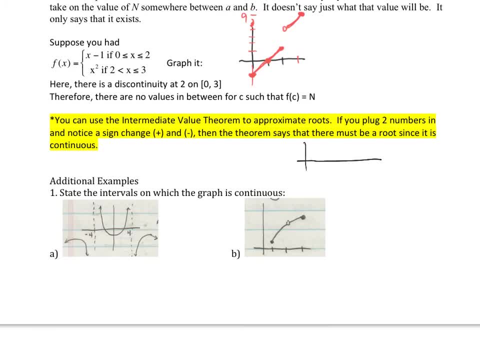 I'm going to draw the y-axis here, And I could draw the y-axis- It doesn't really matter, because right now I'm only concerned with the sign change- And I draw this. I have some sort of continuous function And it has negative values here. 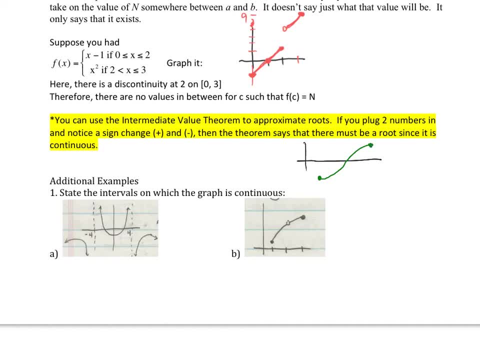 Then it values change to positive And it's continuous. Well, if the values are negative there and the values are positive here, what is in between a negative and a positive? A zero. So long time ago, And sometimes you will notice it on your calculator. 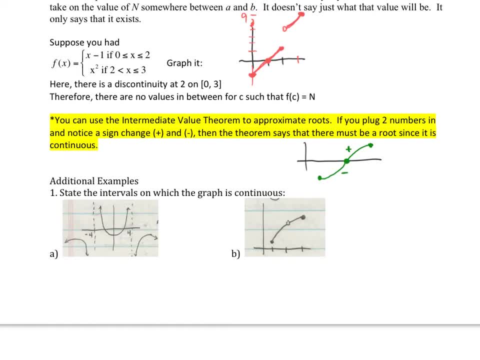 It's just kind of very similar where it asks for the left bound or lower bound, upper bound, when you're trying to solve for those zeros. That's kind of the same situation here. So that's one way that IVT is applicable. You'll see other ways. 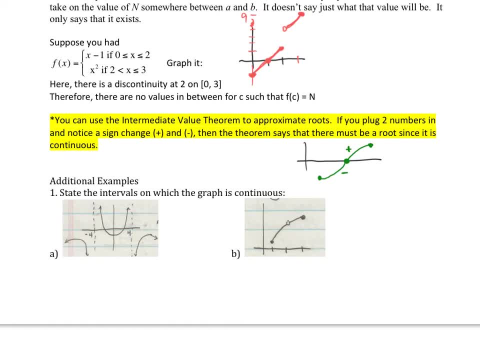 Again, I will show you in class, with some of these examples of how they will appear on the AP test. So that's IVT. So now I'm going to do some select examples And then the ones I'm going to show you are the ones I'm going to show you. are the ones. 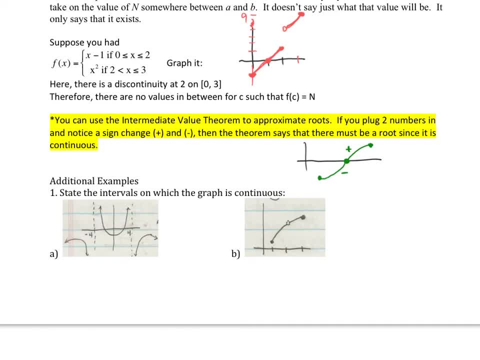 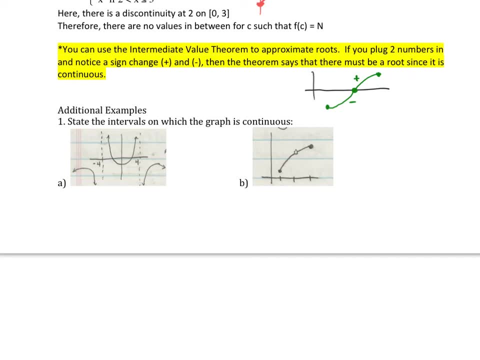 I'm going to show you The ones I don't do here. we could do in class, But let's do a few here. We'll do this first one for continuity state: the intervals on which this function is continuous. Well, looking at this, we can see that it's continuous, right here. 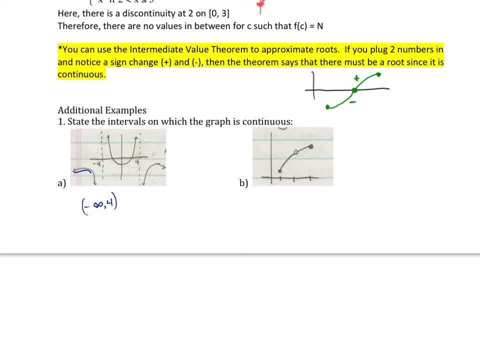 From negative infinity to 4, that asymptote- Then from negative 4 to 4.. And then from 4 to infinity. Looking at the next one Over here, we've got the continuity going from 1, and it's equal to it there- to 2,. 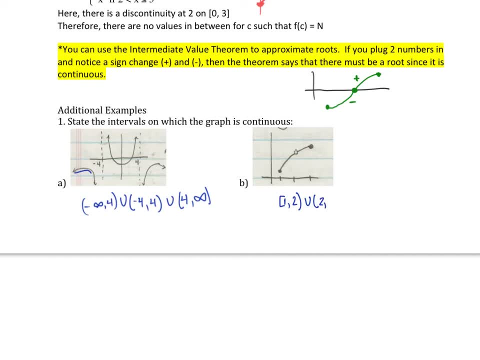 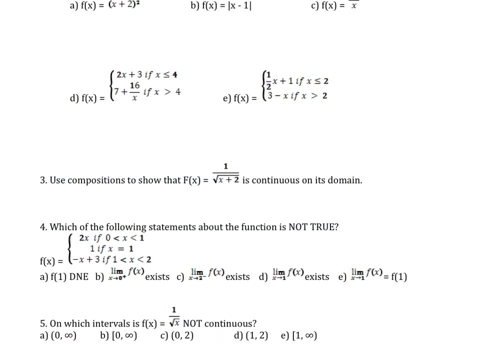 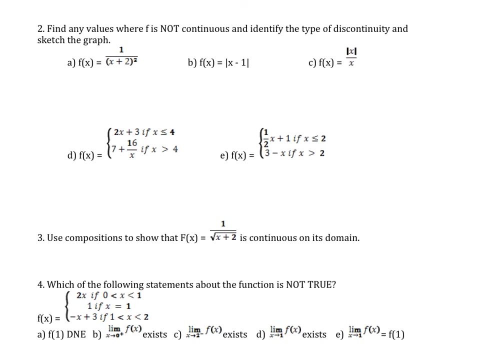 not equal, And then from 2 to 3.. All right, Let's do some of these examples as well. Let's see which ones we will do, And then I will save some for class as well. Let's do number 2.. 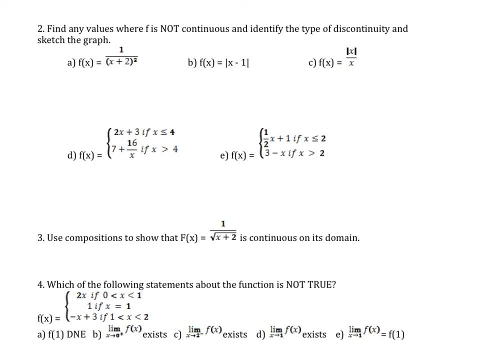 To find Where it's discontinuous And then determine what kind of discontinuity. So for A, if I were to sketch a graph of this, it would look like at negative 2. here there's going to be an asymptote. 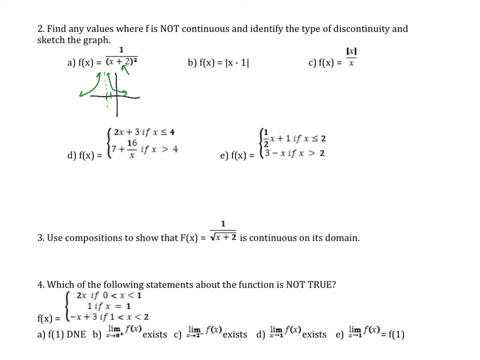 And this side will go up. That side will go up, And I knew that it was at negative 2 because I looked at the graph. This is an infinite discontinuity, Okay, So Continuity At x equals 2.. Okay, 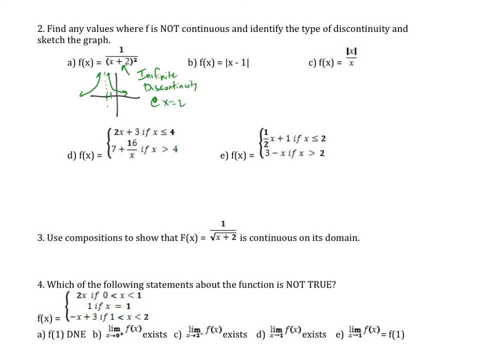 Looking at the next one, Can you see where what it's going to be? It's going to be an absolute value function, All right, So if I were to sketch a quick graph of that- And I'm doing the graph so that you can see it- 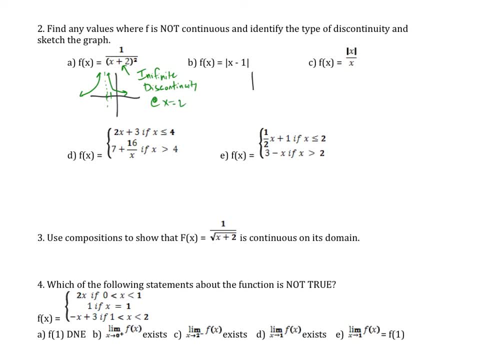 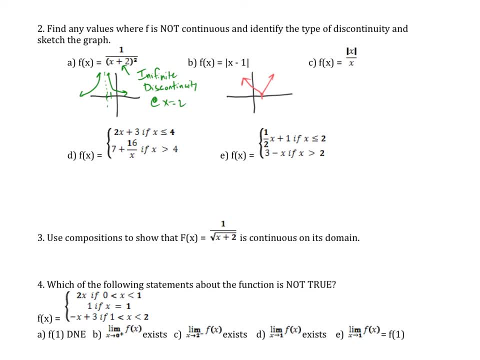 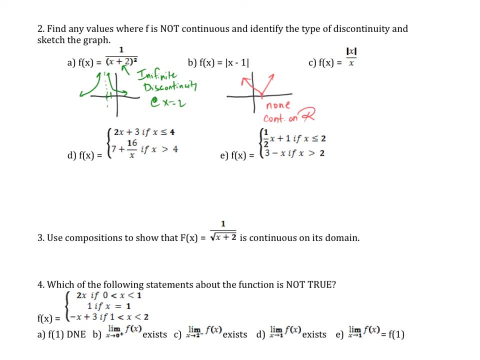 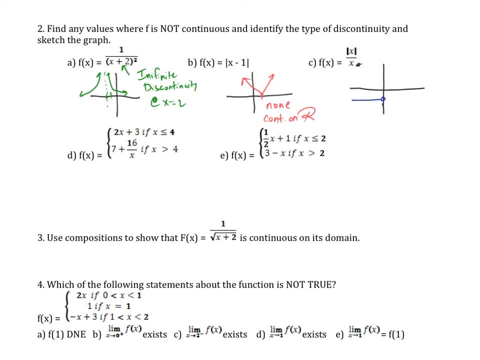 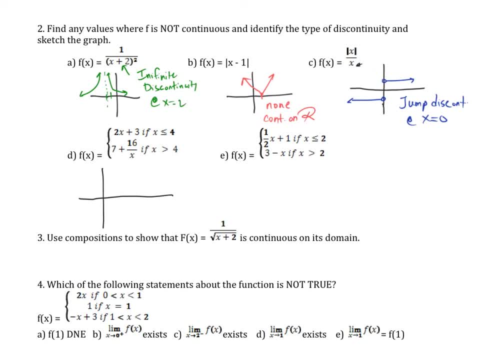 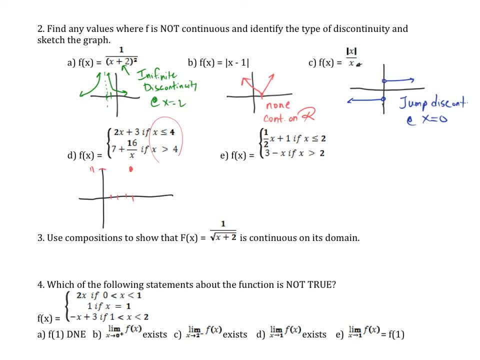 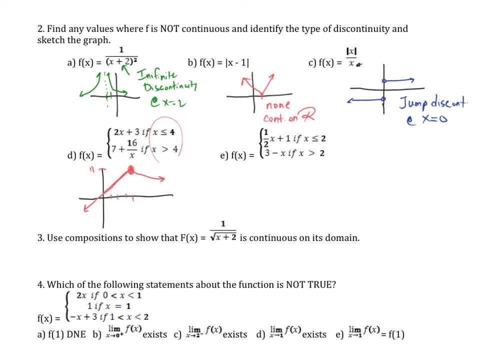 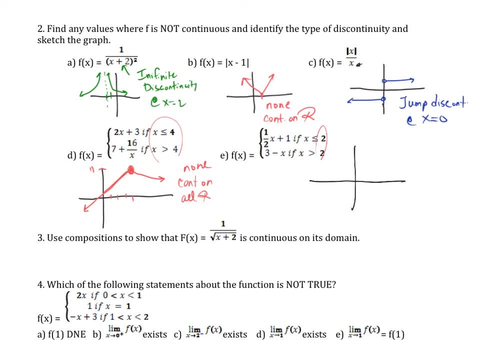 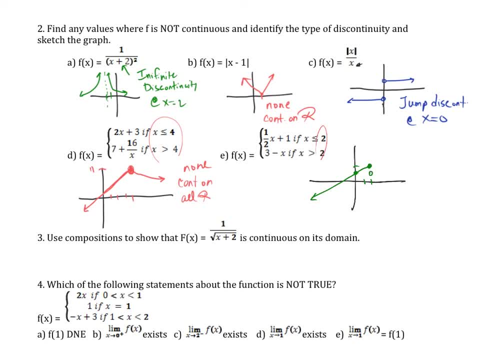 a value of 1, and that'll be an open circle. And then when I put in a value of 3,, I'll get a 0, and that will look like this. So this ends up being a jump discontinuity. So 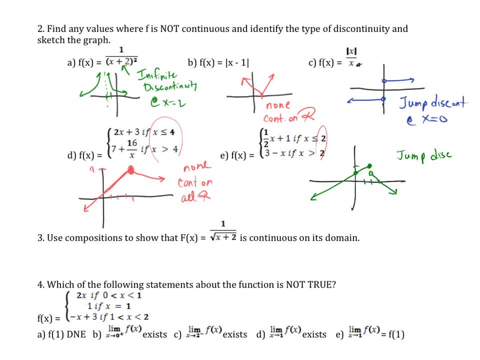 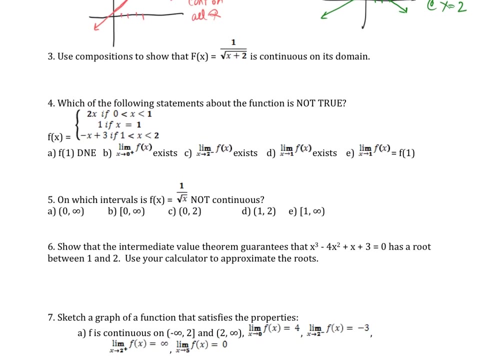 this is a jump discontinuity, You can also call it a non-removable, And this is at. x equals 2.. Let's do one more. Let's skip over and see if we could do an IVT problem right here. Let's do this one, and then we'll save the rest for class. So on this one, it says: 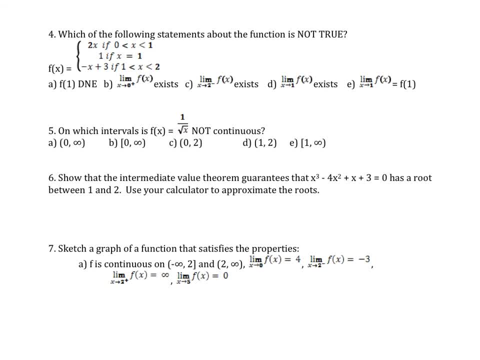 show that the intermediate value theorem guarantees that x, cubed minus 4x, squared plus x plus 3 equals 0, has a root between 1 and 2. Use your calculator to approximate these roots. Okay, so they're telling us that we want to show that it has a root somewhere. 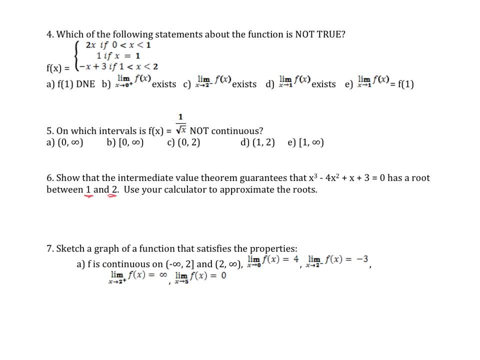 Somewhere between this value 1, and this value 2.. All right, so let's see how we can do this. Let's plug in 1.. It even says use your calculator. So I'm going to plug in f. 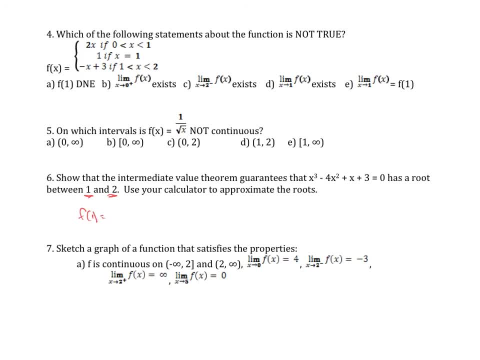 of 1.. F of 1 comes out to be 1 cubed, which is 1, minus 4 times 1,, which is 4, negative 4, plus the 1, plus the 3.. Let's put that 1 in And this comes out to be 1,. but I'm more concerned with it's a positive. 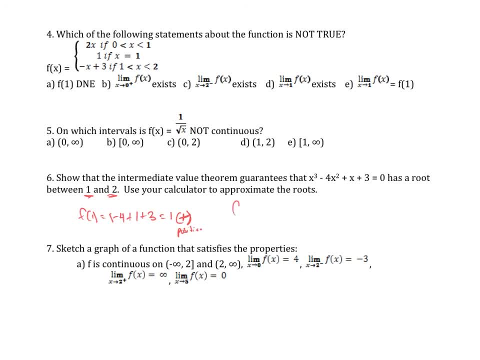 number Positive. Okay, let's try f of 2.. F of 2 is going to give me 8 minus 16, plus 2, plus 3.. And this comes out to negative 3, which is a negative number If I go from. 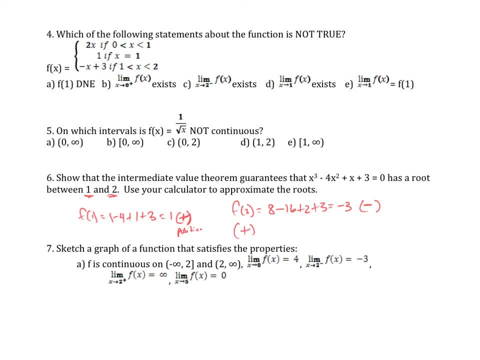 negative to positive. so in this case it's positive, Negative to negative. therefore a sign change on a continuous function. Thus, by IVT there will be a root, There will be a 0 somewhere on there, Because we showed f of 1.. 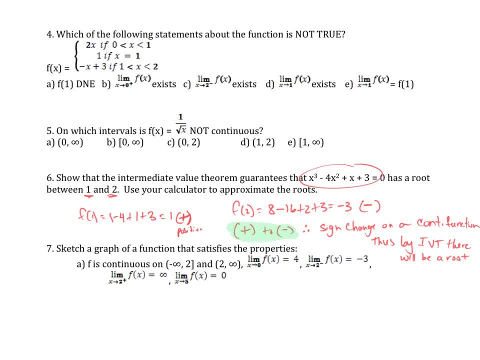 the sign change. Alright. so the sign change right here guarantees that there's going to be a zero somewhere and that's a root Alright. so let's just do one more. I really want to do this one because this is good for the video. 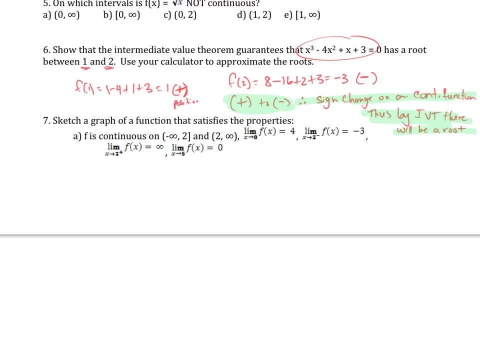 and I'm sure many people outside of my class have questions on things like this. So this is something you will see. on an AP test, You're going to be given all this information. Which of the following represents one of these graphs? So let's see if we could do it where we just have to graph it ourselves. 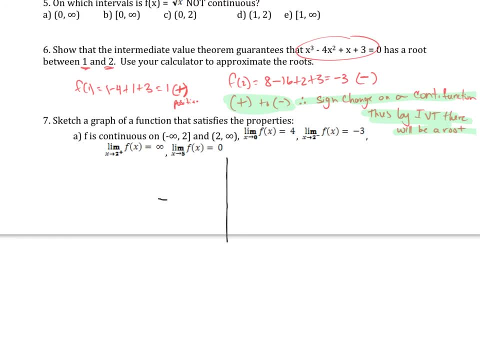 So sketch a graph of the function and I'm going to put an axis here and here's the information I'm given That it's continuous from negative infinity to 2, and then from 2 to infinity. So I know something right away based on this info. happens 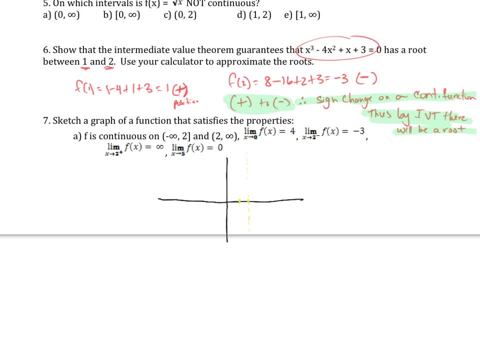 at 2.. And I'm just going to put this. It doesn't necessarily have to be an asymptote, but I'm just going to put that just so that it helps me to remember something's happening at 2 with the continuity. All right. so then I take a look at the next thing, and it says the limit as x goes to. 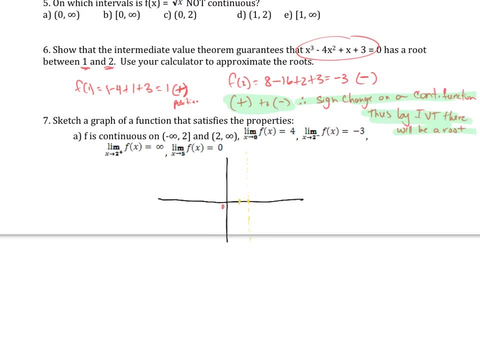 0,. here's my 0. right here is 4.. So that means from the left and from the right, there is a value right here at 4, since that's the limit. Okay, then the limit as I go to 2,, here's 2, from the left-hand side. so that means: 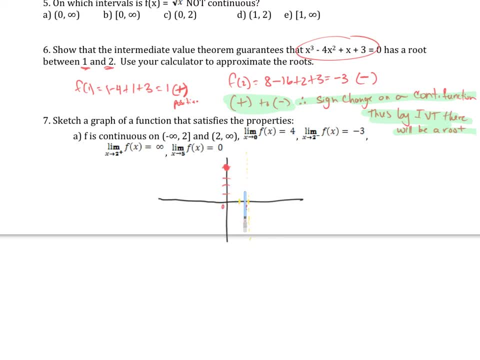 I'm looking at it from here. this limit is going to be negative 3.. Okay, so, just from the left it's negative 3.. So that's 1, 2, negative 3, right here. there is a value there because from the left-hand, 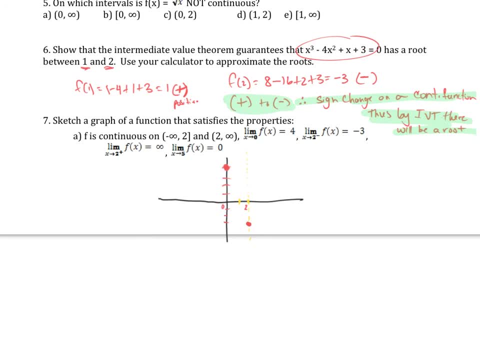 side, I'm reaching that negative 3, and I know that there is a value there because it's closed right here. If that wasn't closed I wouldn't have a value there, So it's continuous from here to here. so that means there is a value there. at 2 from: 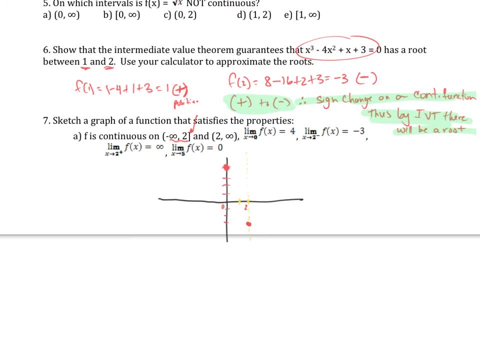 the left and that value is going to be negative. 3, that's where it's approaching. Okay, then, 2 from the right is infinite. so that means it's up here. infinite means it's up there. 2 from the right. 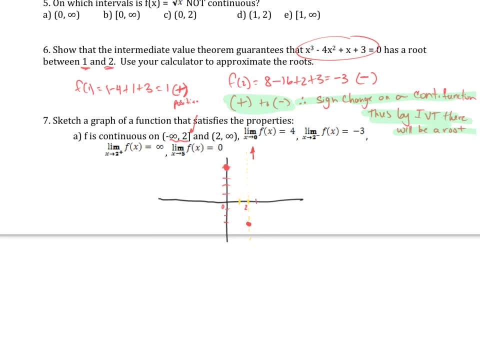 And then the limit, as x goes to 5, is 0, so 1,, 2,, 3,, 4,, 5, it comes all the way down here in 0, and it's continuous, so it's got to cut through this. 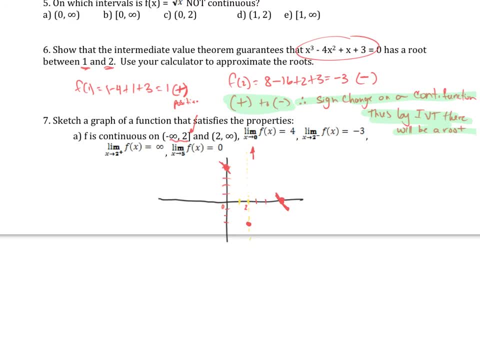 So this has got to cut through here. This has got to cut through here because obviously it's continuous. So now, any way you sketch this could be different, because we don't know what happens in between. I'm going to kind of keep it simple and I'm just going to say this comes down here and 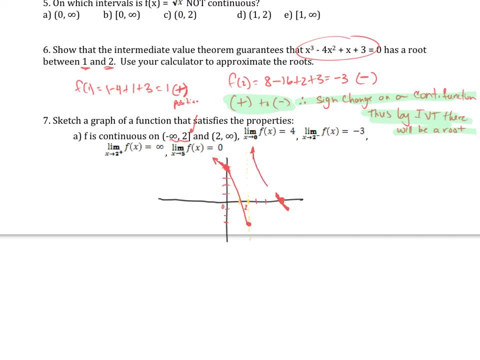 it's going to continue on this way, This will go like this and it'll just continue on that way Again, answers can vary on that, but I'm just trying to keep it as simple as possible. All right, we will stop with that example. we've got many more. we'll take care of them. 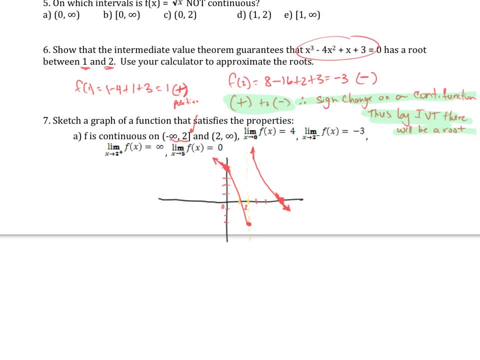 in class. So thanks for watching the video. hit that like and subscribe button and I'll see you guys in the next video. 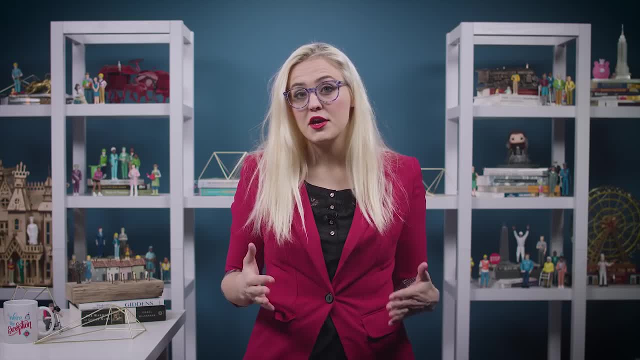 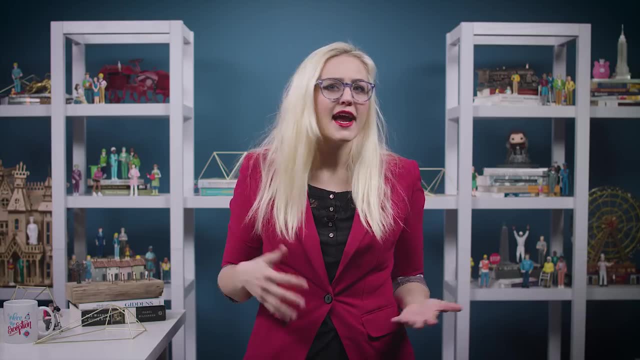 How do you define race? If you had to describe why you think you're a member of one race and someone else was a member of a different one, you'd probably focus on appearances – your skin, your hair, maybe even the structures of your bodies and faces. 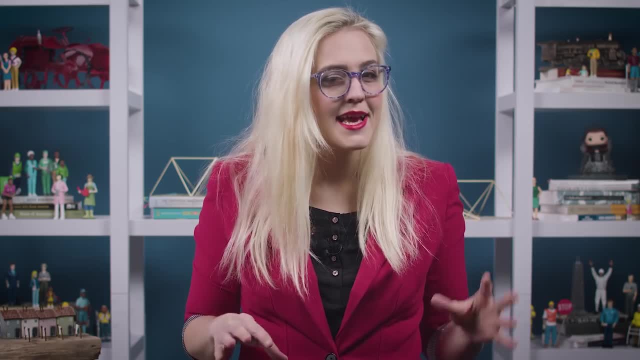 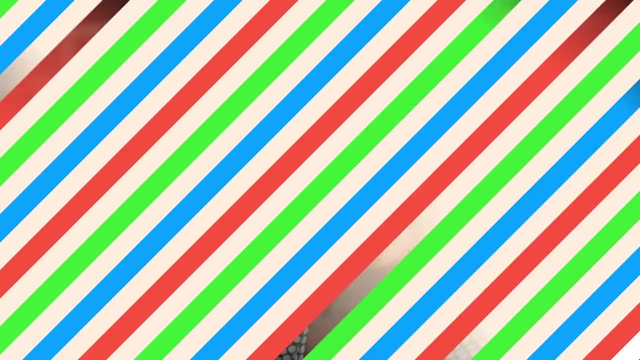 But most of the time those physical criteria mean different things depending on the culture you're a part of. An obvious example is skin color. We use the words white and black to describe two races, but the distinction in skin color between those races isn't as clear cut. 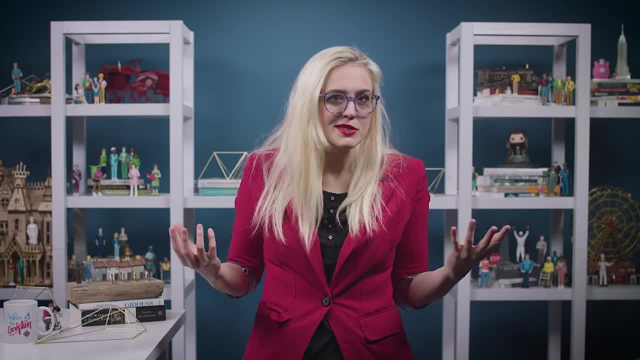 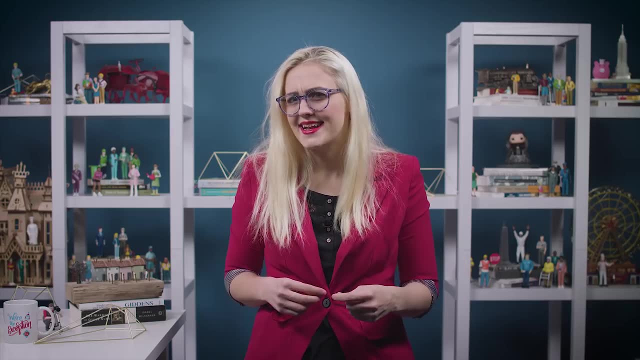 A white person who's spent the summer at the beach might come home with brown skin, but getting a tan doesn't change their race, And light-skinned black people may have skin that's not all that darker than that tan. Clearly, race is about more than just the literal color of someone's skin. 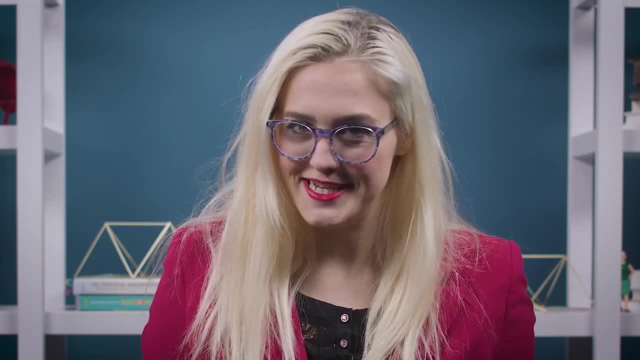 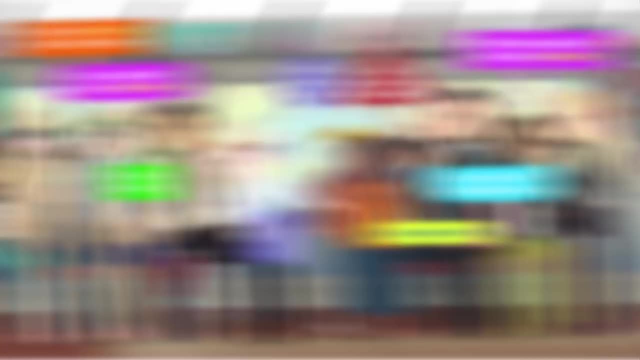 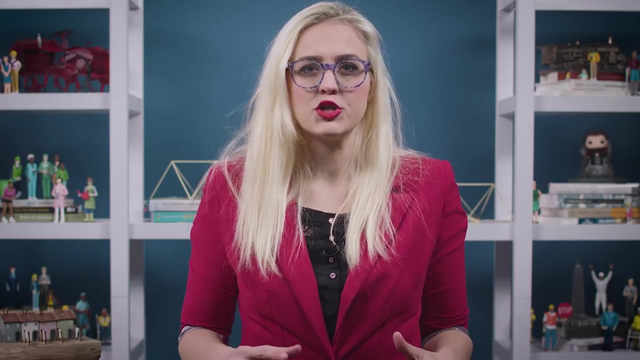 So let's talk about race and why it's a topic that goes more than skin deep. Much like gender, race is a socially constructed category. In this case, it's used to categorize people who share biological traits that a society thinks are important. 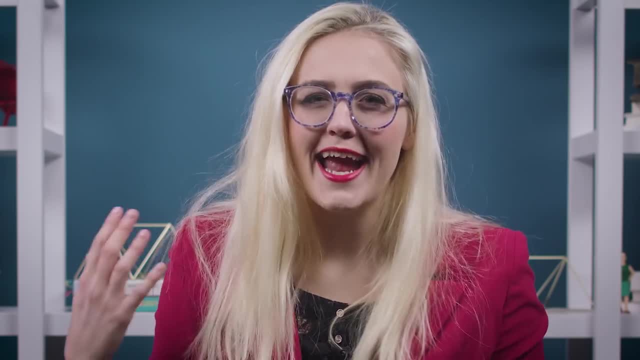 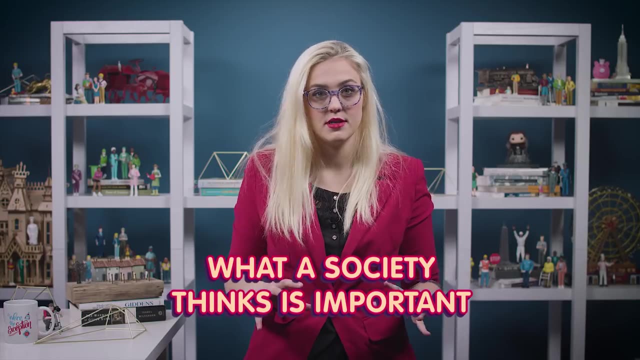 So you might be wondering: how can race be both a social construct and something based on biology? Well, the key part of that definition of race is the last part – what a society thinks is important. Sure, skin color varies widely across regions of the world, but so does eye color.